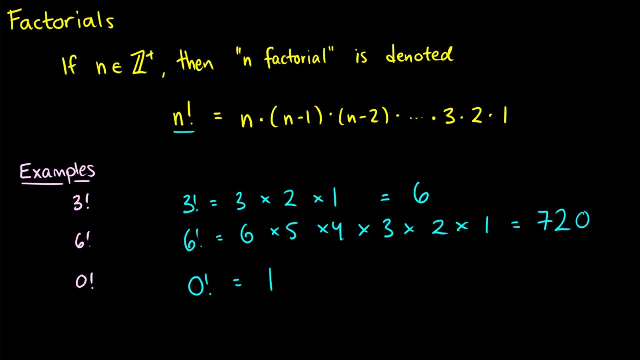 So we can also think of factorials as an example of permutations. So 3 factorial would be the number of ways to arrange 3 objects. 6 factorial is the number of ways to rearrange 6 objects. So here's that example. 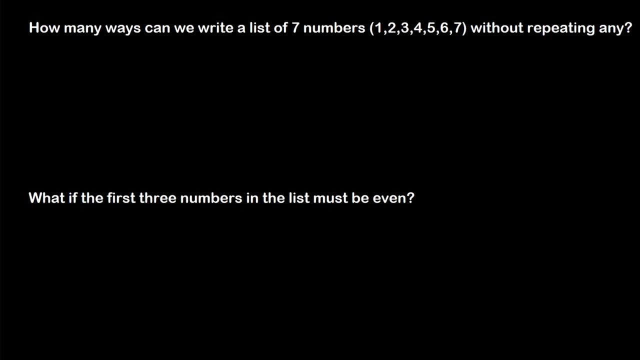 How many ways can we write a list of 7 numbers? so 1,, 2,, 3,, 4,, 5,, 6,, 7, without repeating any? Okay, so that means that for the first number, if we want to pick, we can pick any of the 7, so we have 7 choices for the first number. 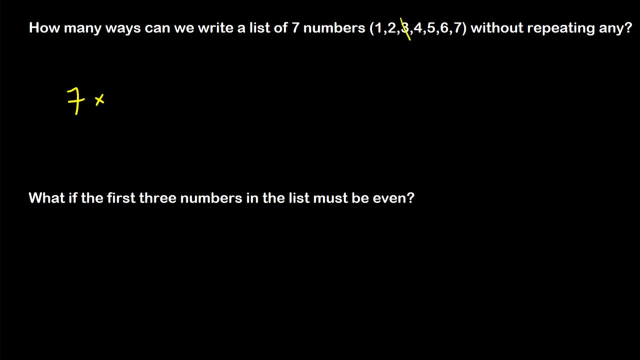 For the second number, let's say we pick 3 as the first number, Then for the second number, we only have 6 choices remaining. So let's say for the second number we pick 6.. Then for the third choice, we only have 5 numbers remaining. 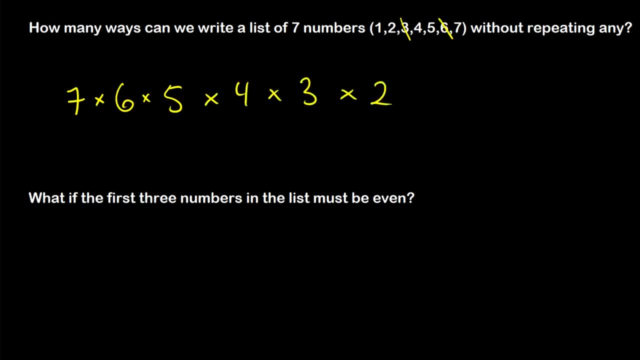 So on and so forth for each subsequent spot. So if we want a list of 7 numbers without repeating any, we have 7 choices for the first slot, 6 for the second, 5 for the third, 4 for the fourth, 3 for the fifth, 2 for the. 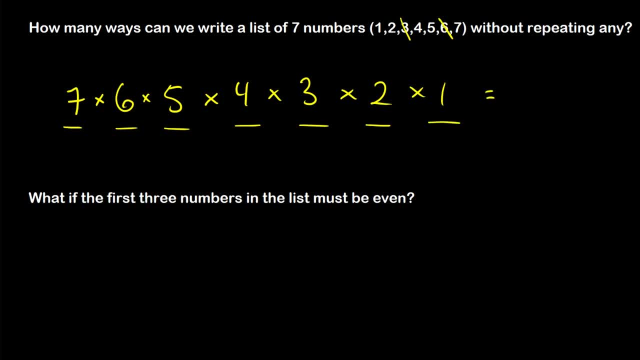 sixth and then 1 for the final slot, Which is the same thing as saying 7 factorial. So ways to rewrite a list of 7 numbers without any repetitions is just 7 factorial. Okay, now what if the first 3 numbers in the list must be even? 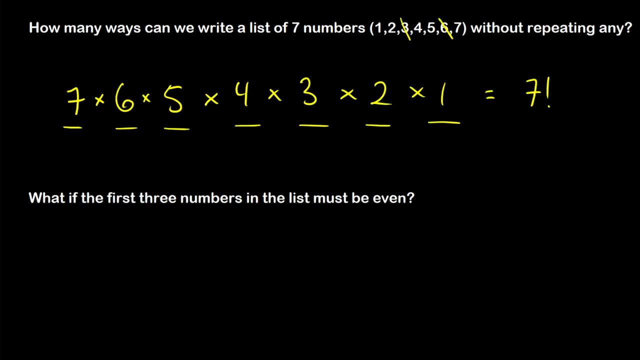 So let's add a condition to this. Okay, so what are the even numbers we have? Well, we have 2,, 4, and 6.. Okay, so for the first number in the list, we have 3 choices, because we have to choose. 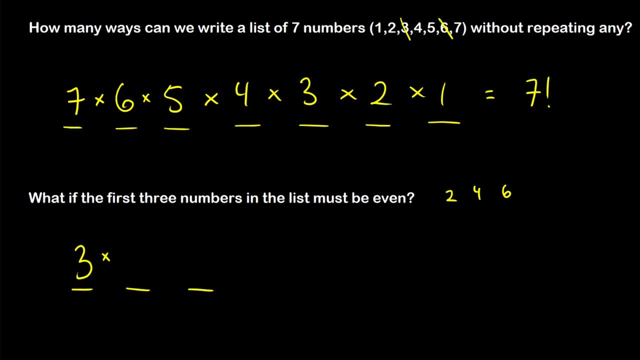 from the first 3 even numbers. So I'm assuming here that we cannot repeat any. So for the second even number then I would have 2 choices remaining. Let's say I pick 4 in the first slot, then I could pick 6 in the second, and then for 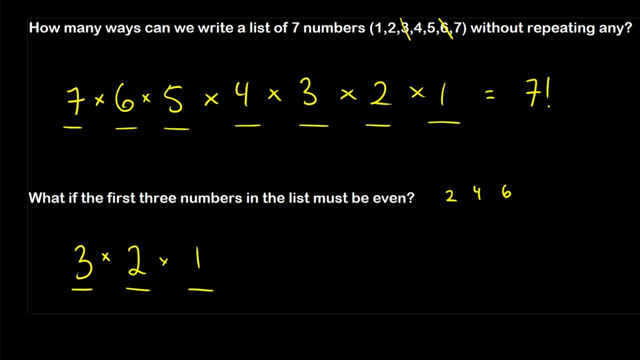 that third slot. I could only pick 2, so I'd only have 1 choice. Okay, So the first 3 numbers had to be even. those are the ways we can fill up the first 3 slots And then for the remaining 4 slots, well, we're left with a bunch of odd numbers. we're left. 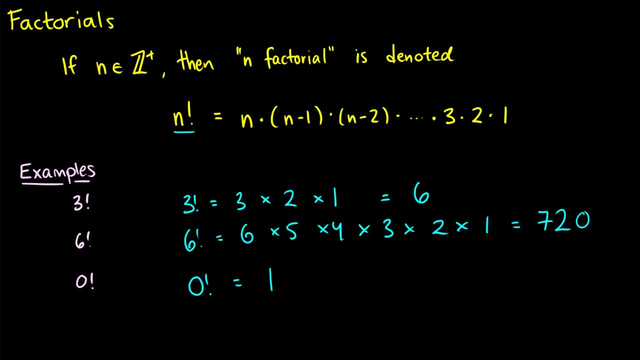 So we can also think of factorials as an example of permutations. So 3 factorial would be the number of ways to arrange 3 objects. 6 factorial is the number of ways to rearrange 6 objects. So here's that example. 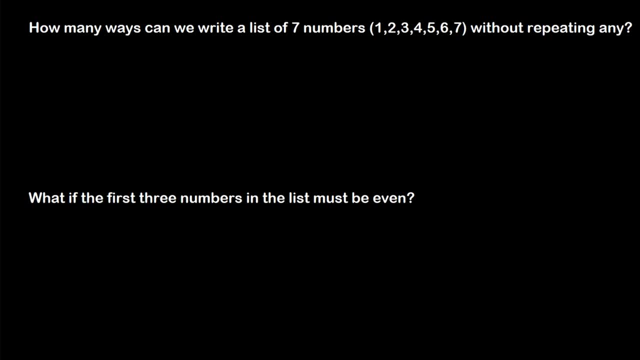 How many ways can we write a list of 7 numbers, so 1,, 2,, 3,, 4,, 5,, 6,, 7, without repeating any? Okay, so that means that for the first number we pick, we can pick any of the 7.. 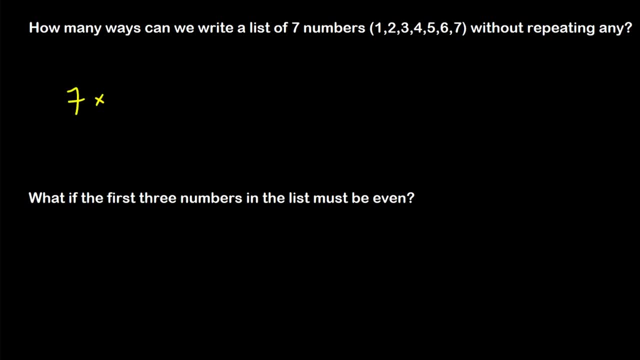 So we have 7 choices for the first number. For the second number, let's say we pick 3 as the first number. Then for the second number, we only have 6 choices remaining. So let's say for the second number, we pick 6.. 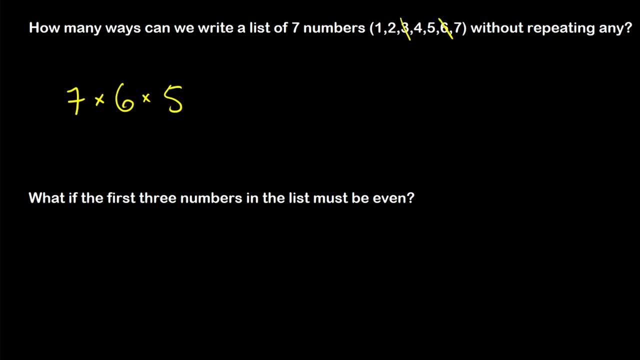 Then for the third choice, we only have 5 numbers remaining, So on and so forth for each subsequent spot. So if we want a list of 7 numbers without repeating any, we have 7 choices for the first slot, 6 for the second, 5 for the third, 4 for the fourth, 3 for the fifth, 2 for the 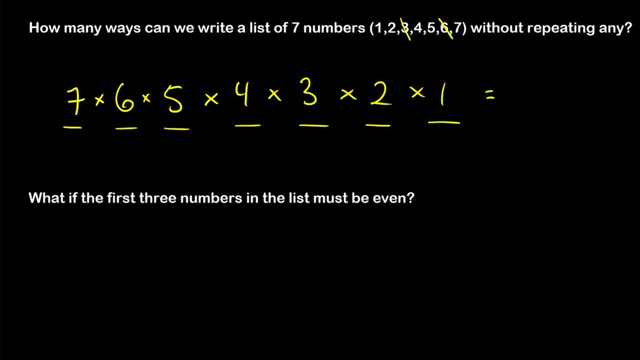 sixth and then 1 for the final slot, Which is the same thing as saying 7 factorial. So ways to rewrite a list of 7 numbers without any repetitions is just 7 factorial. Okay, now what if the first 3 numbers in the list must be even? 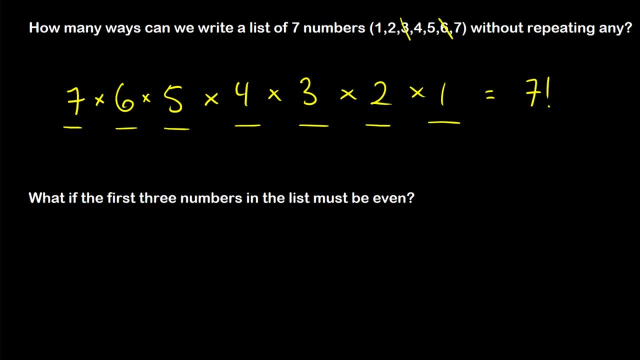 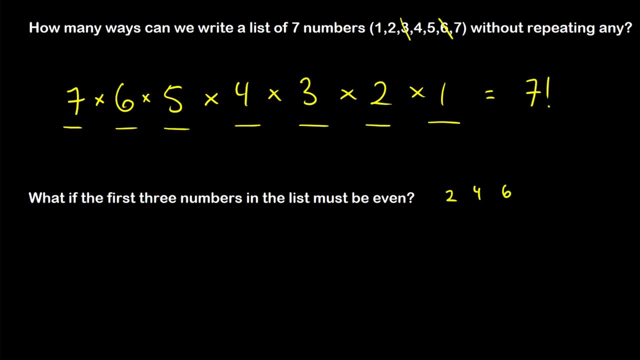 Well, we have 2,, 4, and 6.. Okay, so for the first number in the list we have 3 choices, because we have to choose from the first 3 even numbers. So I'm assuming here that we cannot repeat any. 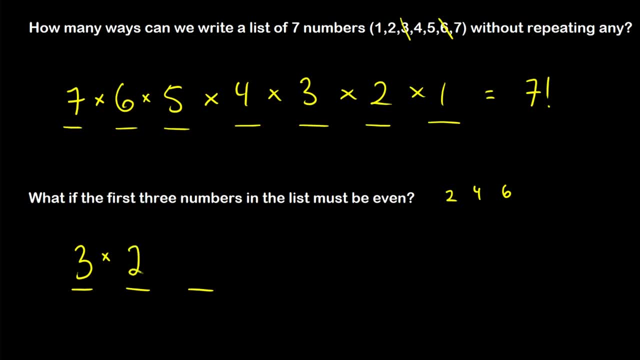 So for the second even number then I would have 2 choices remaining. Let's say I pick 4 in the first slot, then I could pick 6 in the second, and then for that third slot I could only pick 2, so I'd only have 1 choice. 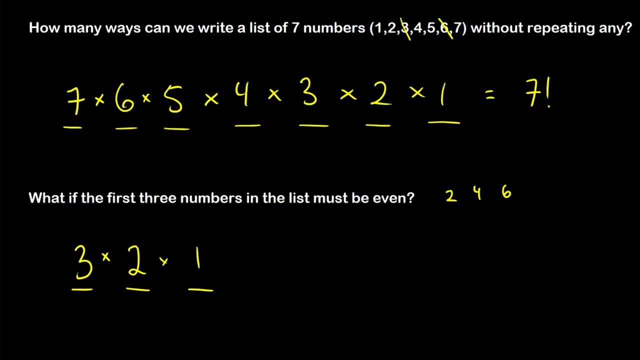 Okay, so the first 3 numbers had to be even. those are the ways we can fill up the first 3 slots and then for the remaining 4 slots, well, we're left with a bunch of odd numbers. We're left with 1,, 3,, 5, and 7.. 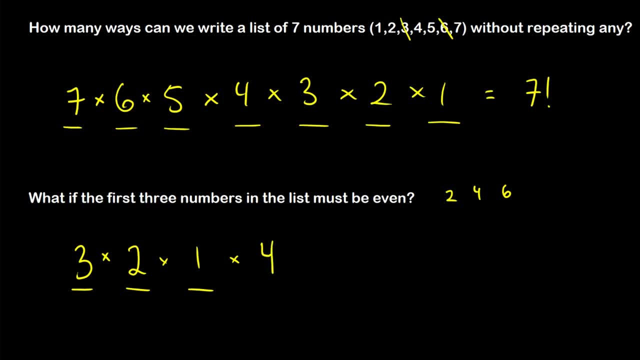 with 1,, 3,, 5, and 7.. So there's 4 choices for the fourth position, 3 choices for the fifth position, 2 choices for the sixth position and 1 choice for the final position. So here we get an answer of 4 factorial times, 3 factorial. 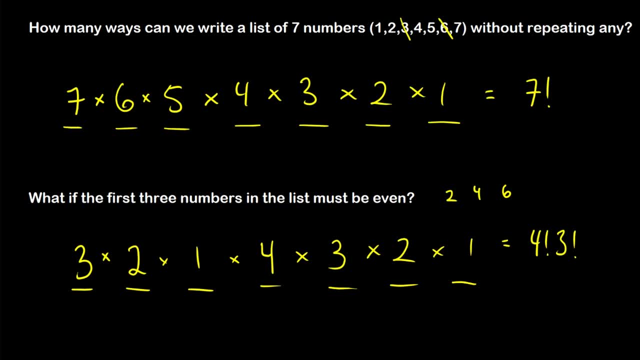 Hmm, Okay, So when we have conditions, sometimes we have to break these problems down into steps. So in the first question we could have whatever number we want in any position, So we could have 7 choices for the first. But in the second problem we have these first 3 positions, which have to be even, and then 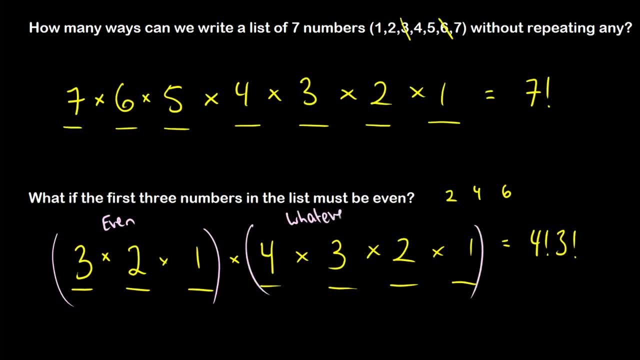 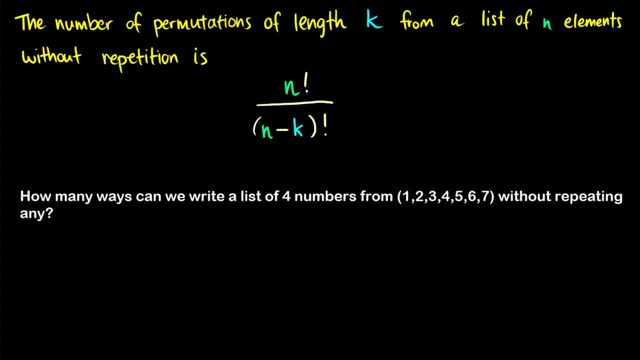 the remaining positions can be whatever. So we did have to look at our even options first And then we could fill in with the remainder. Okay, So when we did that, what we did was we picked from the entire list. So we took 7 items and we rearranged all 7 of them. 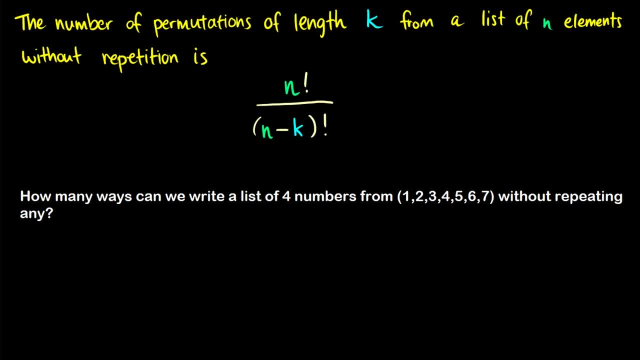 Well, what if we want less than 7 items? So what if we have a list with n things but we only want k of them? So, for example, what if we want 7, like a list of 7 items and we want to pick 4 from? 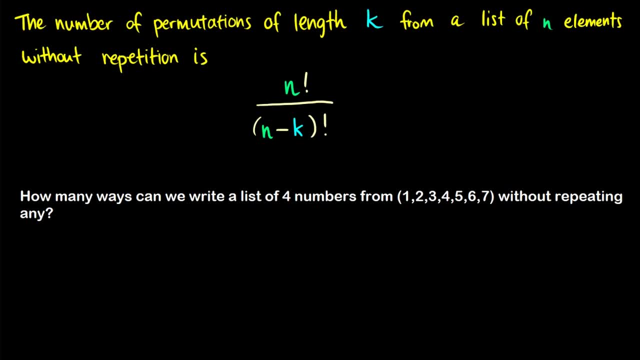 a list of 7?? So it'll be the same problem as before. For the first slot, we have 7 possible choices. For the second slot, we have 6 possible choices. For the fifth slot, or sorry, for the third slot, we have 5 possible choices. 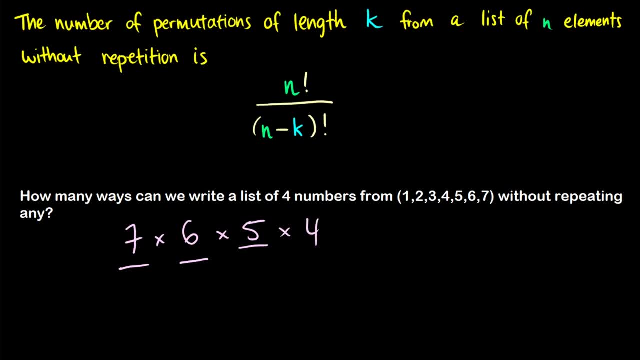 And for the fourth slot, we have 4 possible choices. Okay, So this is how we pick 4 numbers from a list of 7 without repeating any. Now, what's this formula at the top here? Well, this formula: Okay. 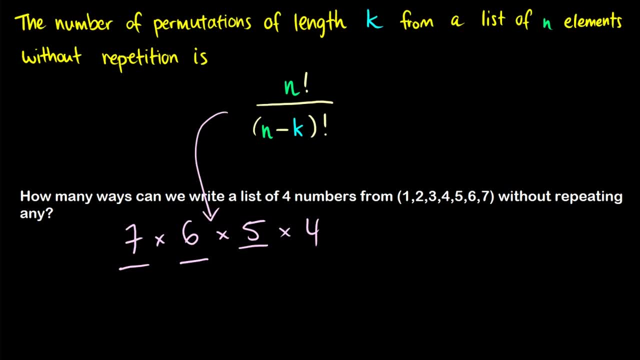 It's the same thing as what we have written down here, So let's rewrite this problem in terms of this formula. So n is the number of elements in the list. So we have 7 items in the list, so let's replace n with 7.. 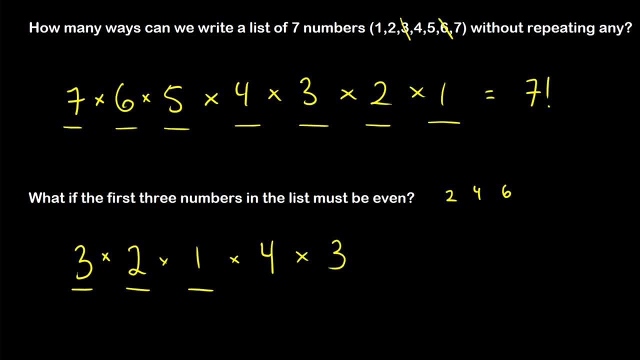 So there's 4 choices for the 4th position, 3 choices for the 5th position, 2 choices for the 6th position and 1 choice for the final position. So here we get an answer of 4 factorial times, 3 factorial. 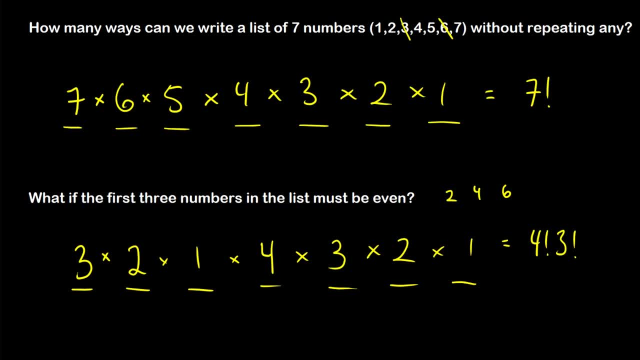 Hmm, okay, So when we have conditions, sometimes we have to break these problems down into steps. So in the first question we could have whatever number we want in any position, so we could have 7 choices for the first. but in the second problem we have these first 3 positions. 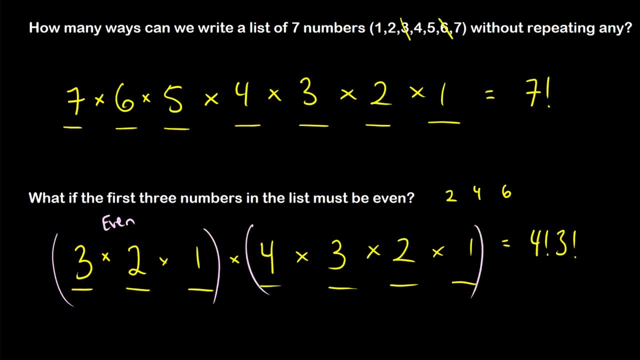 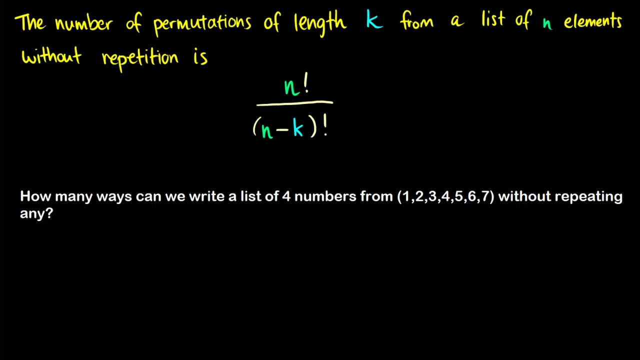 which have to be even, and then the remaining positions can be whatever. So we did have to look at our even options First, and then we could fill in with the remainder. Okay, so when we did that, what we did was we picked from the entire list. 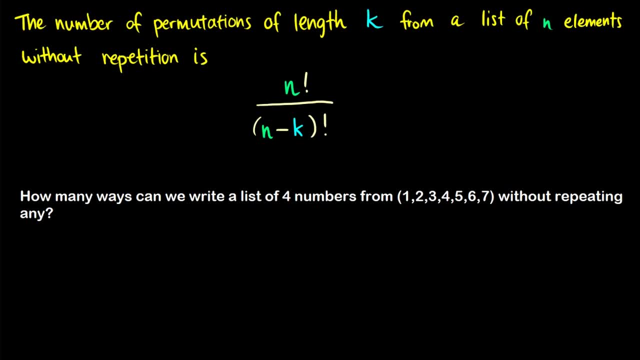 So we took 7 items and we rearranged all 7 of them. Well, what if we want less than 7 items? So what if we have a list with n things but we only want k of them? So, for example, what if we want 7, like a list of 7 items- and we want to pick 4 for? 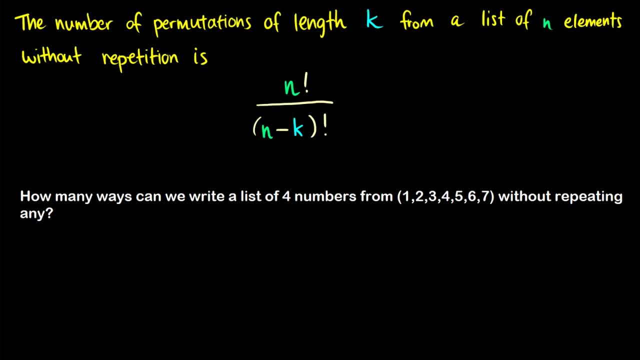 from them. So it'll be the same problem as before. For the first slot, we have 7 possible choices. for the second slot, we have 6 possible choices. for the fifth slot- or sorry, for the third slot, we have 5 possible choices and for 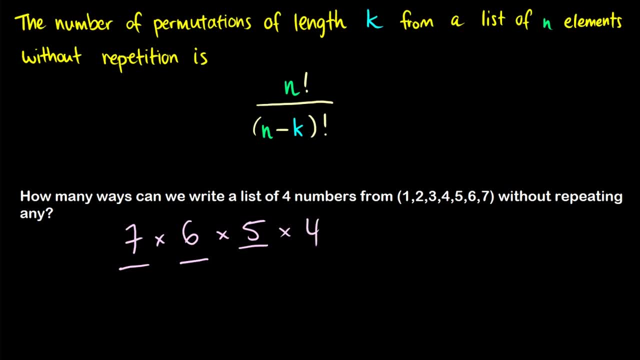 the fourth slot, we have 4 possible choices. Okay, so this is how we pick 4 numbers from a list of 7 without repeating any. Now, what's this formula at the top here? Well, this formula is the same thing as what we have written down here. 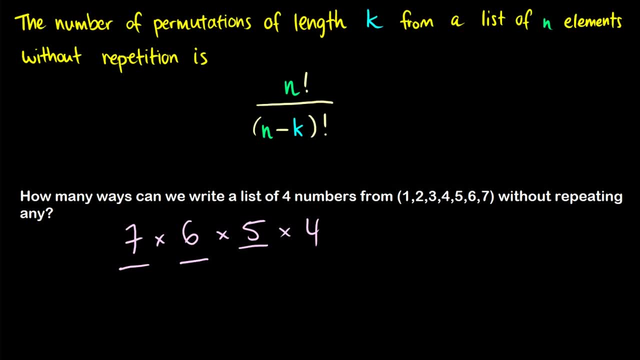 So let's rewrite this problem in terms of this formula. So n is the number of elements in the list, So we have 7 items in the list, so let's replace n with 7.. Okay, so we want to pick k of them. 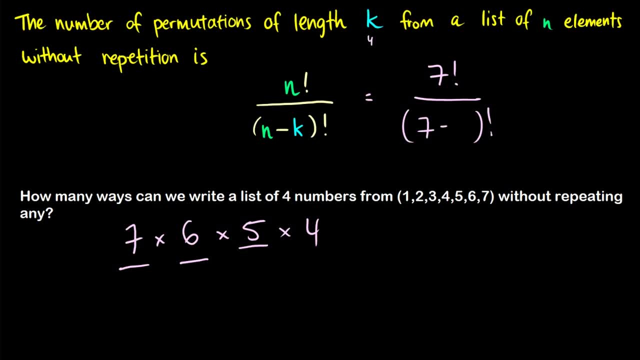 So we're going to subtract. well, we're picking 4,. 4 is equal to k in this case. so this is 7 factorial over 7 minus 4 factorial. Now this is equal to 7 factorial over 3 factorial. 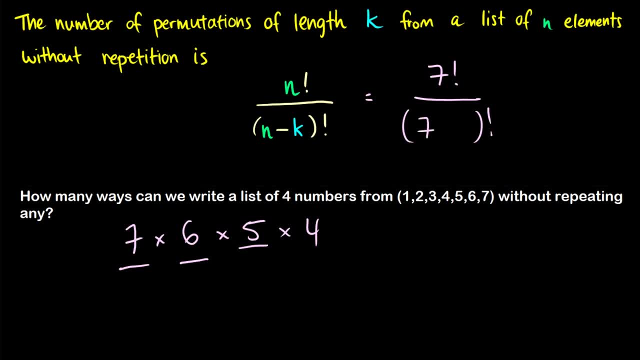 Okay, So we want to pick k of them. So we're going to subtract: Well, we're picking 4.. 4 is equal to k in this case, So this is 7 factorial over k Over 7 minus 4 factorial. 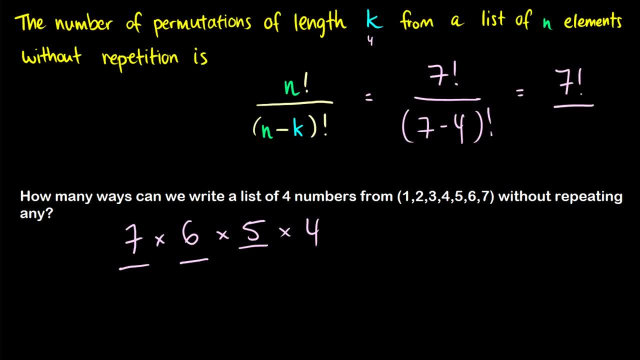 Now, this is equal to 7 factorial over 3 factorial. So how are these two equivalent? Well, let's take a look at the math. What is 7 factorial over 3 factorial? If we expand this out, this is 7 times 6 times, 5 times 4 times 3 times 2 times 1.. 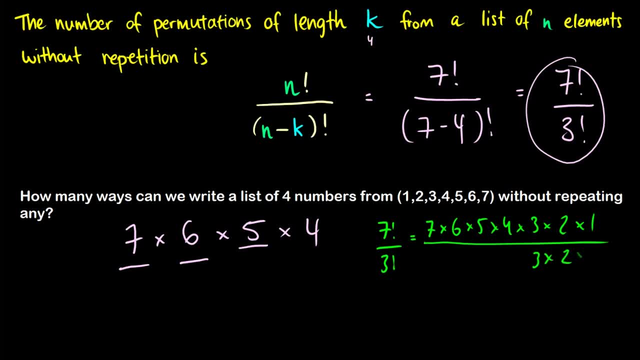 Okay, 3 factorial is 3 times 2 times 1.. Now these all cancel, So what we're left with on the top is 7 times 6 times 5 times 4, which is exactly what we have on the left side. 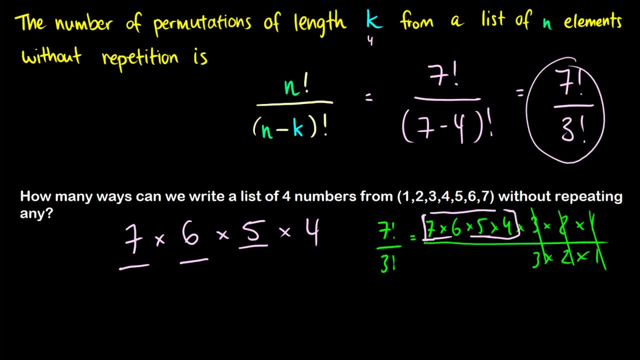 Okay, So if we just take the formula n factorial over n minus k factorial, we can just plug in some numbers and get a result, Or we can do it in the same method, where we count each case and we end up with the same result. 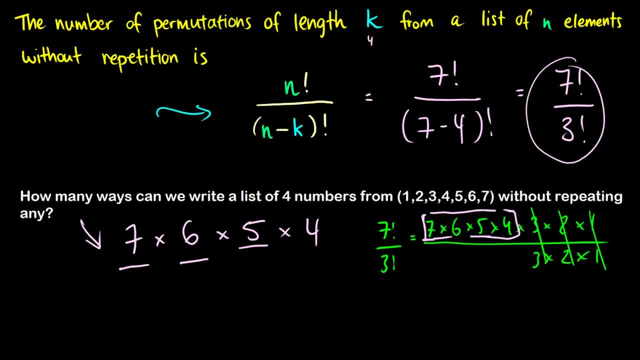 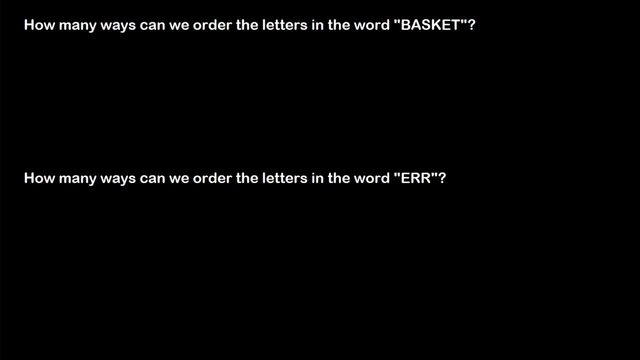 Of course, the formula is a lot faster and is essentially a derivation that we can take from all of these examples. Okay, Now what if we don't use numbers? What if we try to disguise these questions as word problems? For instance, how many ways can we order the letters in the word basket? 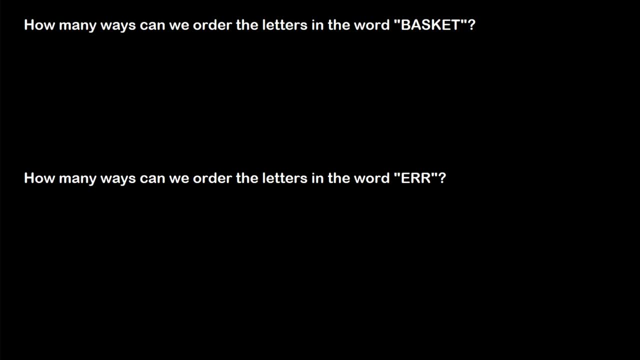 Okay. So here we have B-A-S-K-E-T, We don't have any repeating letters, So why don't we just assign these letters numbers, Okay: 1, 2, 3,, 4,, 5, 6.. 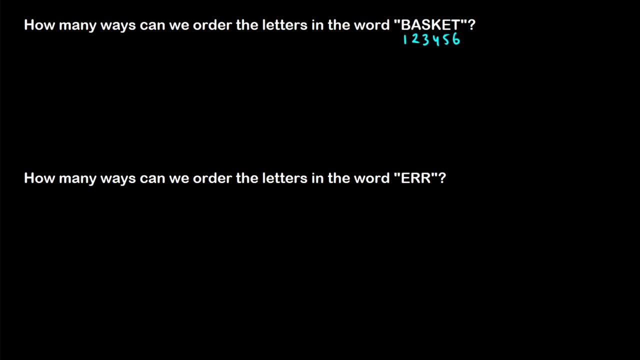 So how many ways can we order the letters in the word basket is really the same thing as asking how many ways can we rearrange the numbers in the list: 1, 2, 3, 4, 5, 6.. So we know this is just going to be 6 factorial. 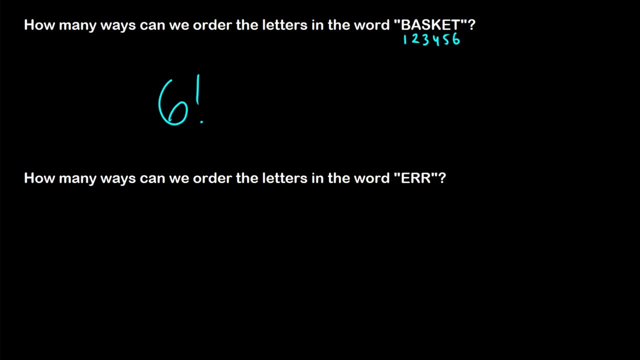 There's 6 choices for the first slot, 5 choices for the second slot, 4 choices for the third slot, and so on. Okay, What about this? How many ways can we order the letters in the word air? Okay? 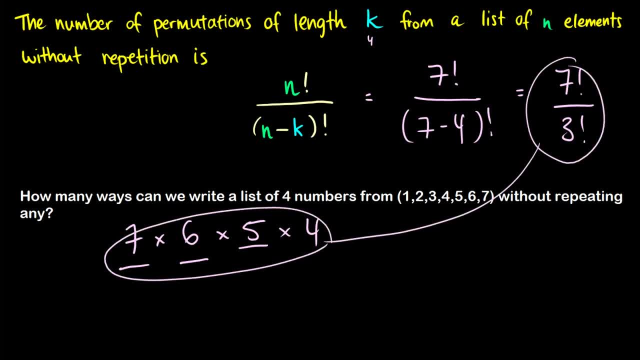 So how are these two equivalent? Well, let's take a look at the math. What is 7 factorial over 3 factorial? If we expand this out, this is 7 times 6 times 5 times 4 times 3 times 2 times 1.. 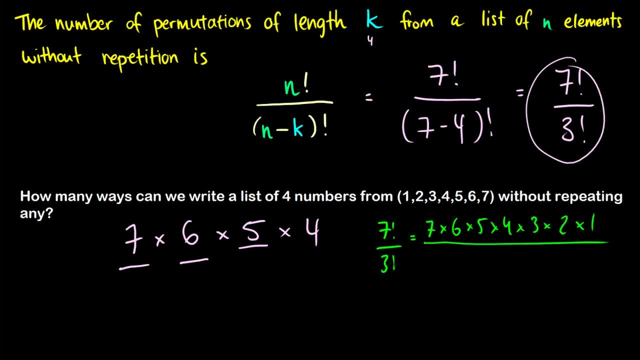 Okay, Okay, 3 factorial is 3 times 2 times 1.. Now these all cancel, So what we're left with on the top is 7 times 6 times 5 times 4, which is exactly what we have on the left side. okay. 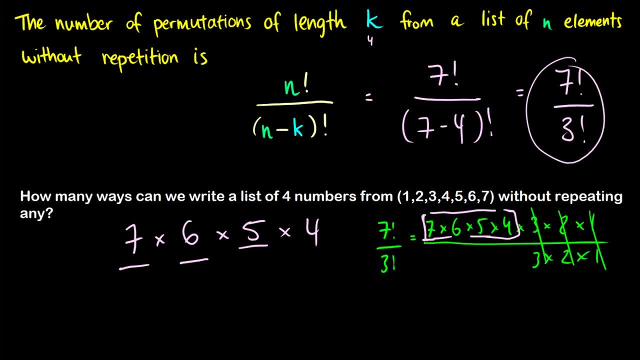 So if we just take the formula n factorial over n minus k factorial, we can just plug in some numbers and get a result, Or we can do it in the same method, where we count each case and we end up with the same result. 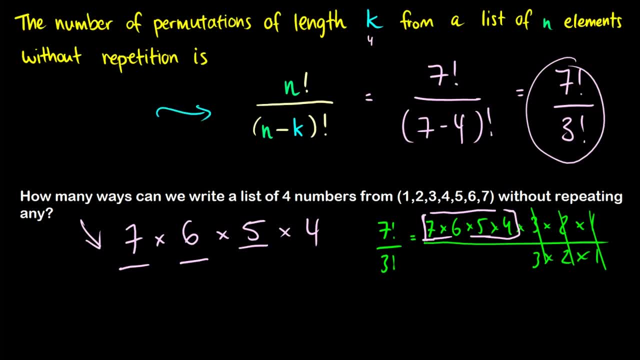 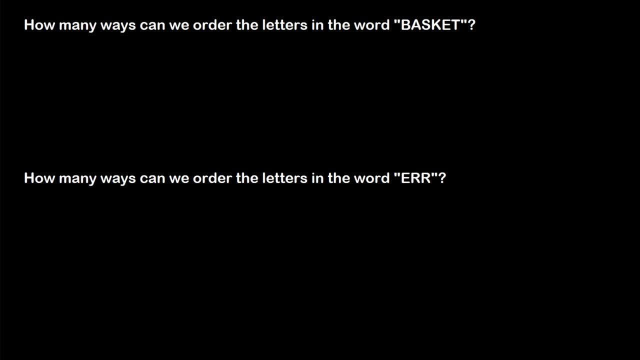 Of course, the formula is a lot faster and is essentially a derivation that we can take from all of these examples. Okay, now what if we don't use numbers? What if we try to disguise these questions as word problems? For instance, how many ways can we order the letters in the word basket? 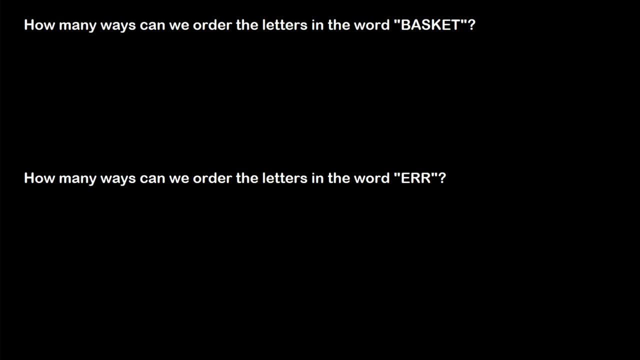 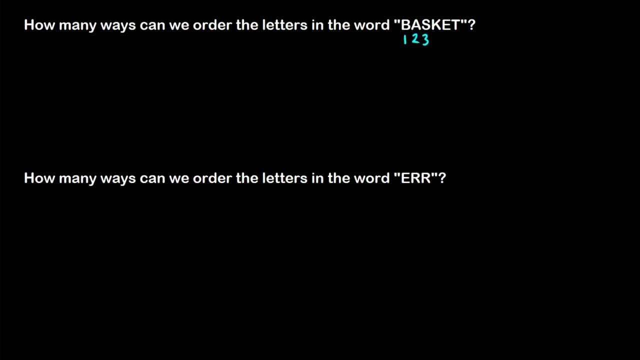 We don't have any repeatable letters. We don't have any repeatable letters. We don't have any repeatable letters. So why don't we just assign these letters numbers Okay, 1, 2,, 3,, 4,, 5,, 6.. 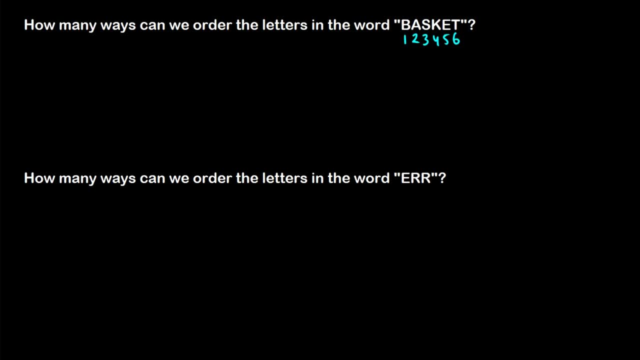 So how many ways can we order the letters in the word basket is really the same thing as asking how many ways can we rearrange the numbers in the list: 1, 2, 3, 4, 5, 6.. So we know this is just going to be 6 factorial. 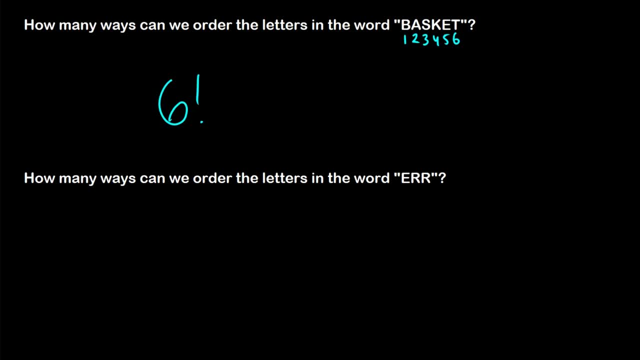 There's 6 choices for the first slot, 5 choices for the second slot, 4 choices for the third slot, and so on. Okay, what about this? How many ways can we order the letters in the word air? Okay, so this is interesting because we have two letters that are the same. 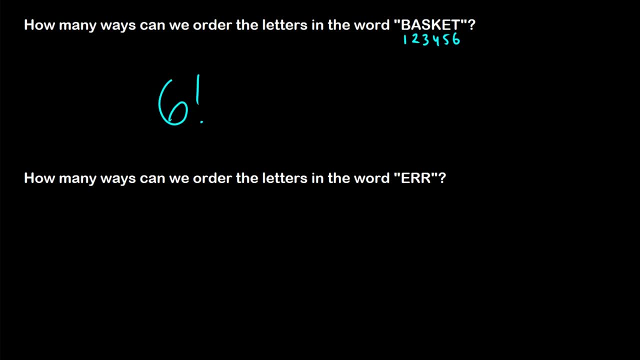 So this is interesting because we have two letters that are the same. This is kind of like having two numbers that are the same. Now, there's an interesting problem here, because if we were just to write all of the different combinations or permutations we have, we could have E-R-R. 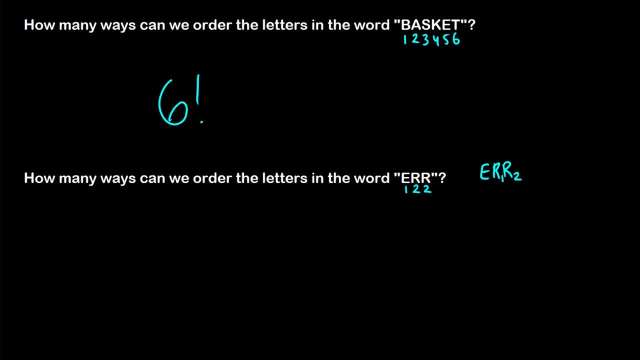 We could have, and actually let's just label these R's explicitly, So the first R is R1.. And the second R is R2.. We could have E-R2 and R1.. So we could flip the R's. We could have R1-E-R2, R1-R2-E. 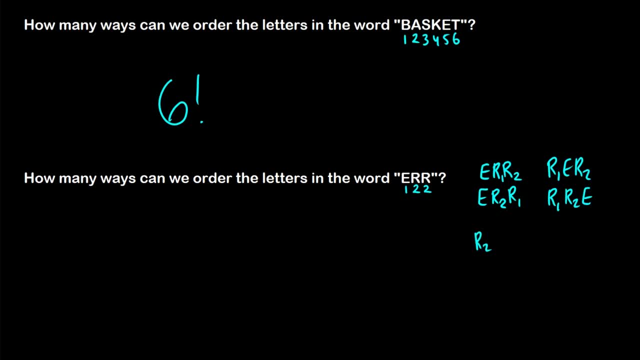 We could also have R2-E-R1.. And we could have R2-E- oh sorry, R2-R1 and E. Okay, Okay, So in total, we think we have six different ways to do this, if we list out all the possible. 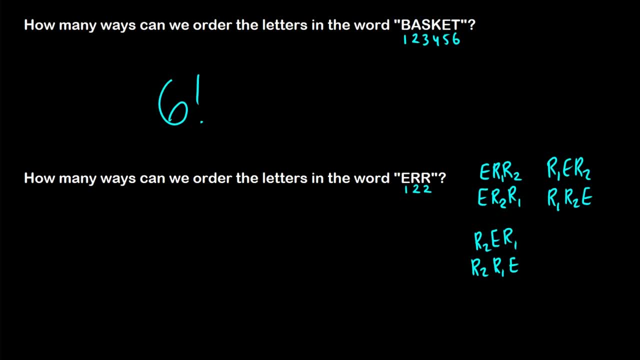 combinations. But what we notice is that, well, E-R1-R2 and E-R2-R1, they're really the same thing, because in words an R is an R. We also see here that R2-R1 and E are pretty much the same thing. 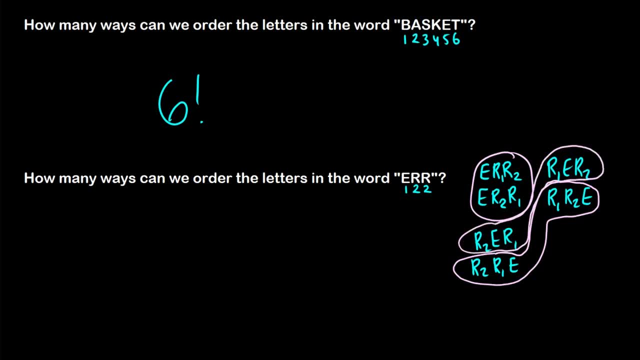 And so is R2-E-R1 and R1-E-R2.. So, really, we don't have six different possible ways to do this, We have three. Hmm, Okay, So what formula can we use here? If we were just to do this regularly, we would say: this is three factorial, because we'd have 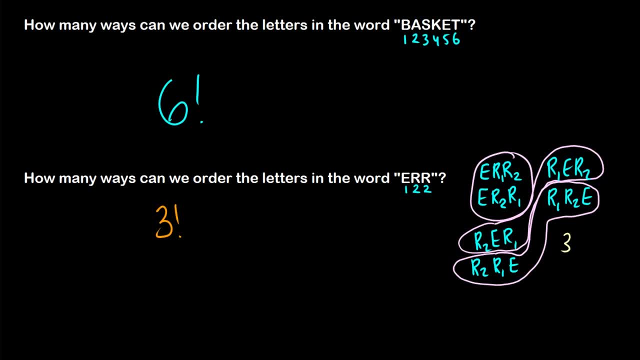 three different things to rearrange, But what we see is that there are some duplicates. So what we can do is we can divide by the number of times every single letter occurs. So This may sound a little interesting. So E-R-R, there's only one way that we can arrange our Es with inside the word. 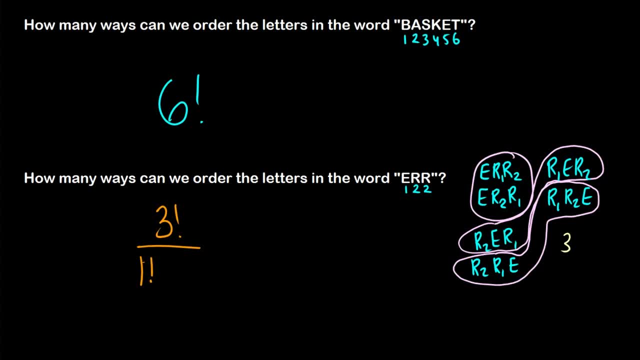 So we divide by one factorial and this really doesn't do anything. But with the R and the R there's two different ways. we can arrange the two Rs in every single case. So we can divide by two factorial, So the one factorial doesn't do anything. so this is just three factorial over two factorial. 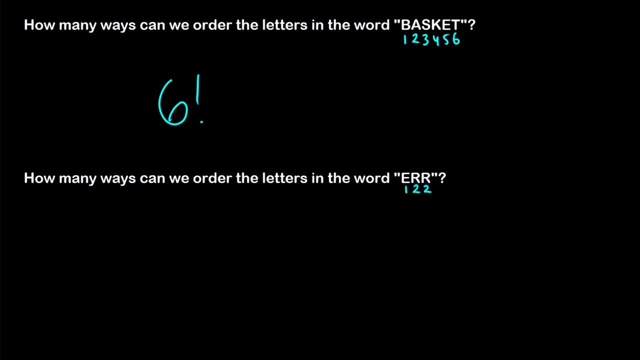 This is kind of like having two numbers that are the same. Now there's an interesting problem here, because if we were just to write all of the different combinations or permutations we have, we could have E, R, R, We could have, and actually let's just label these R's explicitly. 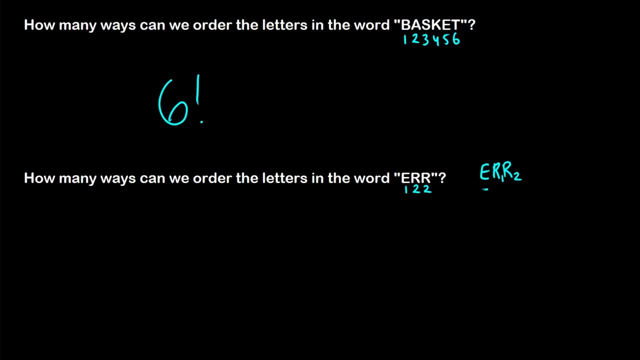 So the first R is R1 and the second R is R2.. We could have E, R2, and R1.. So we could flip the R's. We could have R1, E, R2,, R1,, R2, E. 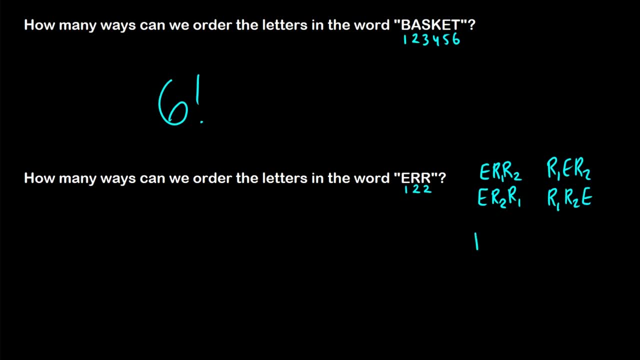 We could also have R2, E, R1, and we could have R2, E- sorry, R2, R1, and E. So in total, we think we have six different ways to do this, if we list out all the possible combinations. 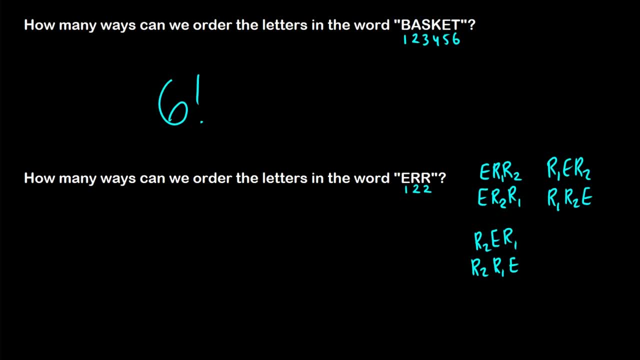 But what we notice is that, well, E, R1, R2, and E, R2, R1, they're really the same thing, because in words an R is an R. We also see here that R2, R1, and E are pretty much the same thing. 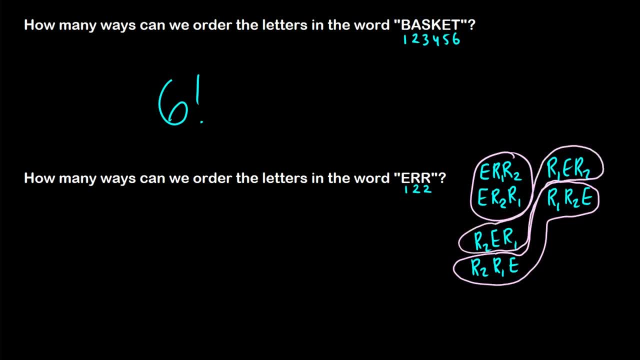 And so is R2, E R1, and R1, E R2.. So really, we don't have six different possible ways to do this, We have three, Okay. so what formula can we use here? If we were just to do this regularly, we would say: this is three factorial. 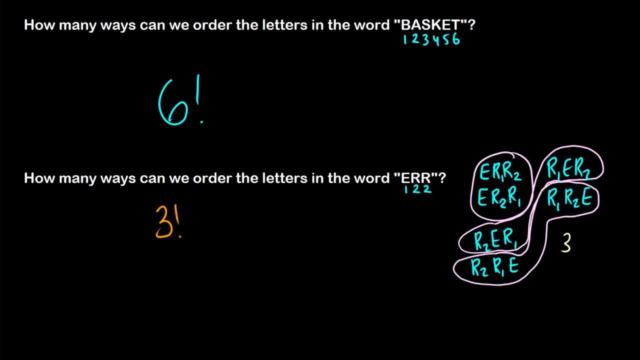 because we'd have three different things to rearrange. But what we see is that there are some duplicates. So what we can do is we can divide by the number of times every single letter occurs. So This may sound a little interesting. So E R R, there's only one way that we can arrange our Es with inside the word. 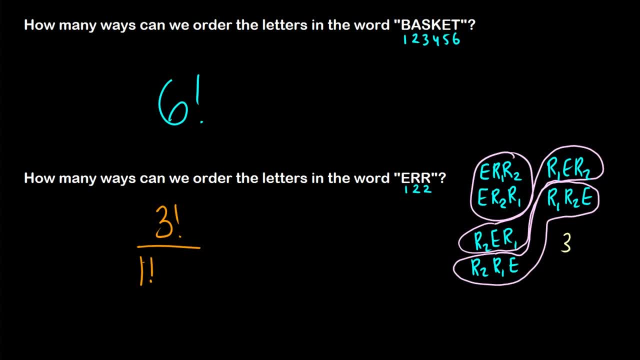 So we divide by one factorial and this really doesn't do anything. But with the R and the R there's two different ways. we can arrange the two Rs in every single case, So we can divide by two factorial, So the one factorial doesn't do anything. 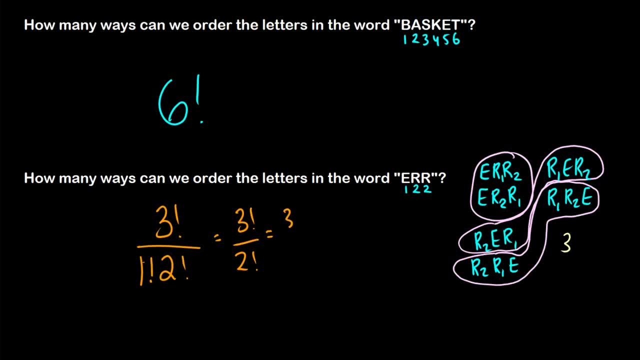 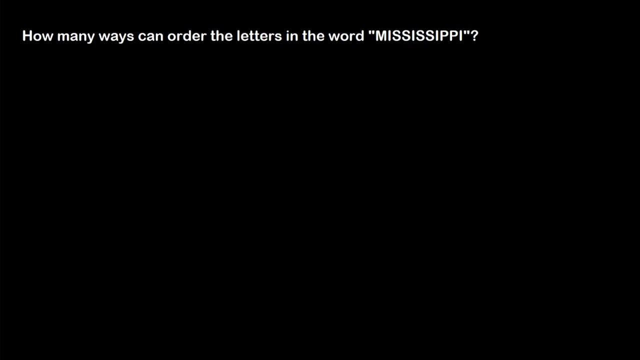 So this is just three: factorial over two factorial, which is three. So we have three times two times one over two times one, and we're just left with three as a result. Okay, let's do a more complicated process, Mississippi. Okay, so we have an M, we have an I, we have two S's, we have another I. 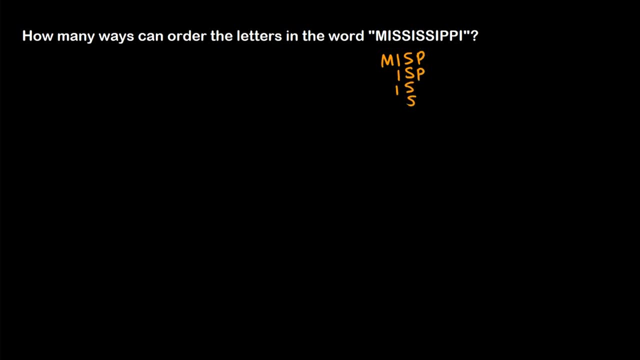 we have another two S's, we have an I, we have two P's and an I. As you can see, I've rearranged the letters in kind of this grid, And what I'm doing in this grid is I'm figuring out how many of each letter occurs. 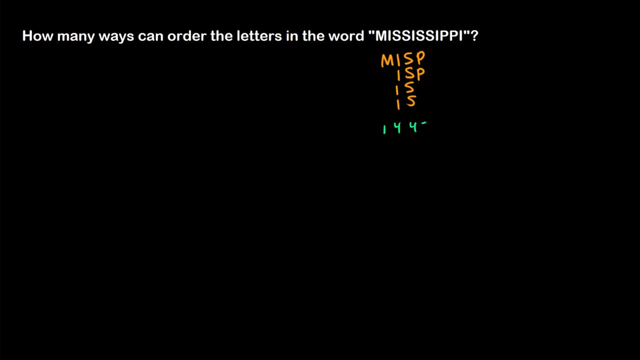 So I know we have one M, four I's, four S's and two P's, If we want to rearrange this. well, how many letters are there in total? One, two, three, four, five, six, seven, eight, nine, ten, eleven. 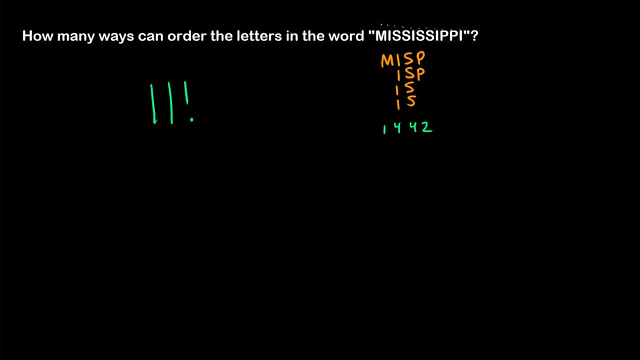 So if we just want to rearrange all of the letters, there's 11 factorial ways of doing this. But we have some repeat letters, which means that if we take, say, S1, S2, S3, and S4, it doesn't matter what order they're in. 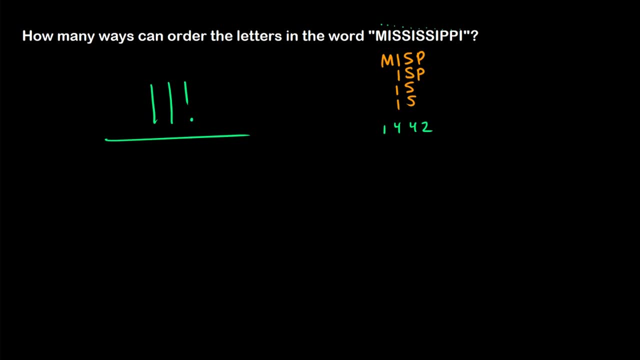 They're all the same. So we divide by the number of similar letters factorial. So if we have one M, we divide by one factorial. If we have four I's, we divide by four factorial. Four S's divide by four factorial. 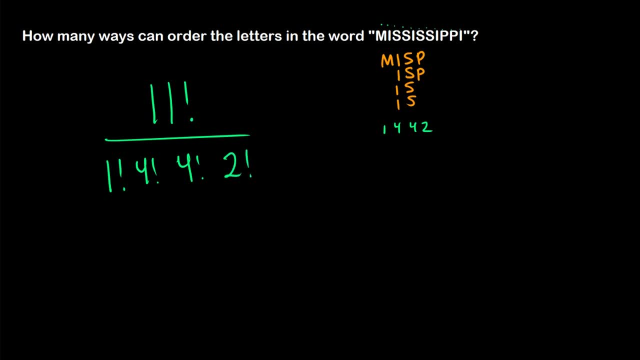 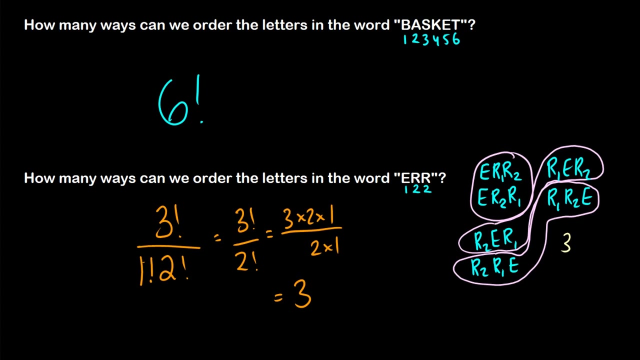 Two P's, divide by two factorial, And this is how many ways we can order the letters in the word Mississippi. Now, the nice thing about this method is that this works for every single case, whether there's duplicate letters or not. Let's look at the first problem with basket. 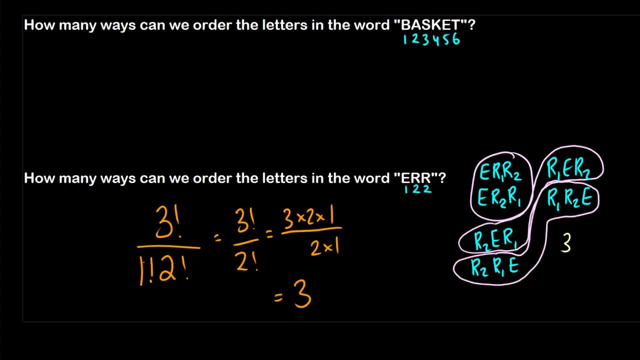 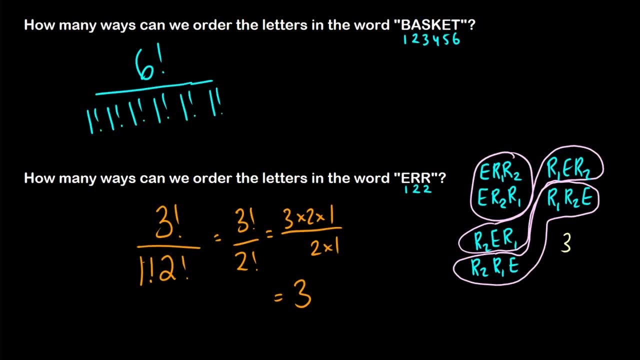 So this is the same method as before, but because we only have one of each, this is just dividing by one. So we have six times. so this is just six factorial. So you can just use this method for every problem, if you wanted to. 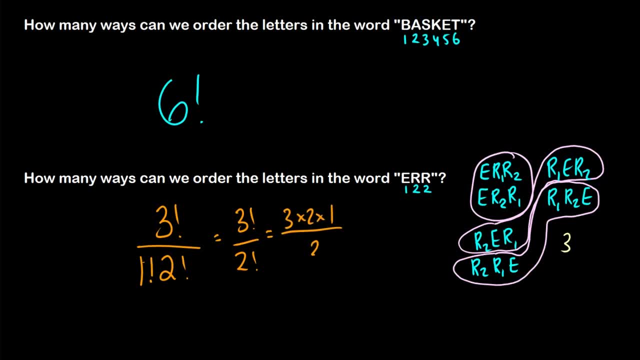 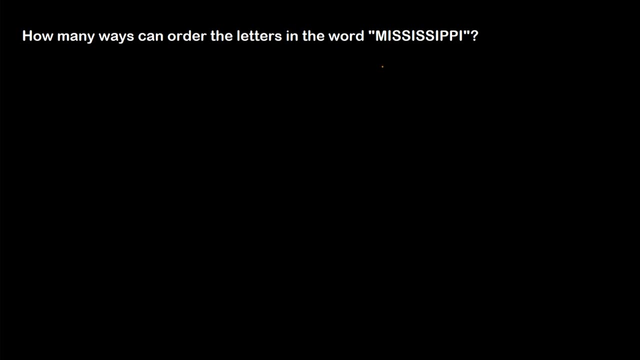 which is three times two factorial, Okay. So that's two times two times one, over two times one, and we're just left with three as a result. Okay, let's do a more complicated process: Mississippi- Okay. So we have an M, we have an I. we have two Ss. we have another I, we have another two. 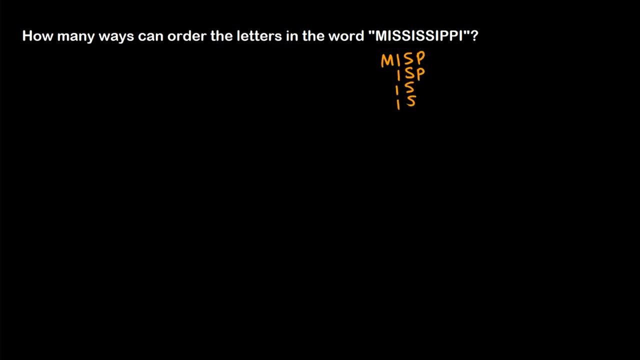 Ss, we have an I, we have two Ps and an I. As you can see, I've rearranged the letters in kind of this grid, Okay. So what I'm doing in this grid is I'm figuring out how many of each letter occurs. 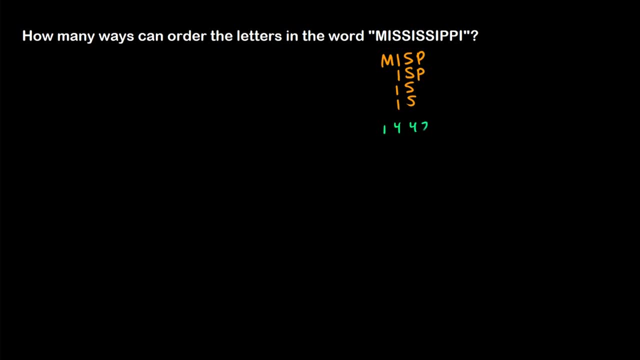 So I know we have one M, four Is four Ss and two Ps, If we want to rearrange this. well, how many letters are there in total? One, two, three, four, five, six, seven, eight, nine, ten, eleven. 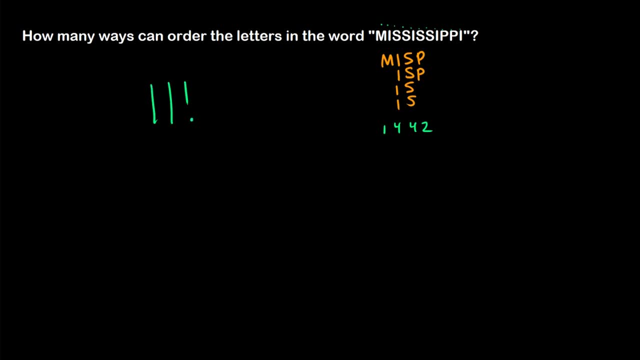 So if we just want to rearrange all of the letters, there's eleven factorial ways of doing this. but we have some repeat letters, which means that if we take, say, S1, S2, S3, and S4. 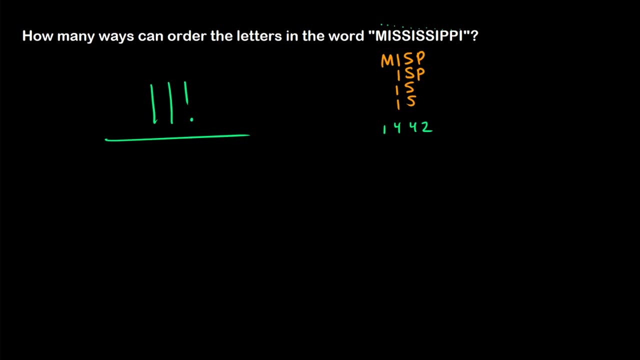 It doesn't matter what order they're in, They're all the same. So we divide by the number of similar letters factorial. So if we have one M, we divide by one factorial. We have four, Is we divide by four factorial. 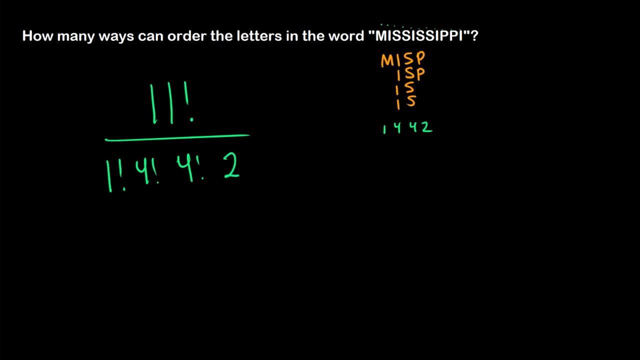 Four Ss divide by four factorial. Two Ps divide by two factorial. And this is how many ways we can order the letters in the word Mississippi. Now, the nice thing about this method Is that this works for every single case, whether there's duplicate letters or not. 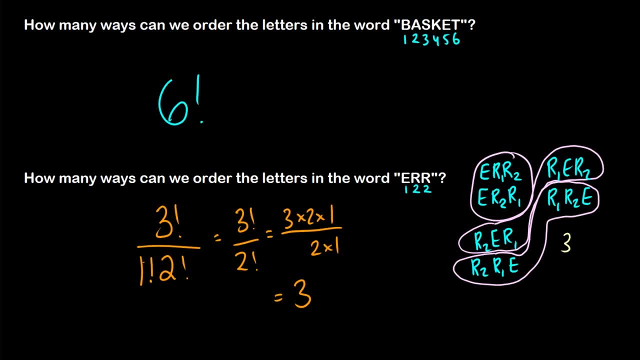 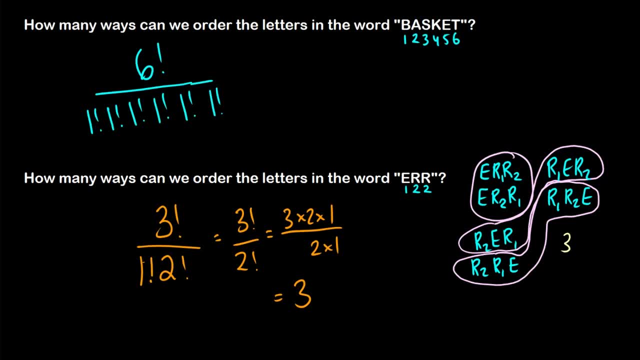 one factorial and one factorial. So this is the same method as before, but because we only have one of each, this is just dividing by one. So this is just six factorial. You can just use this method for every problem, if you wanted to. 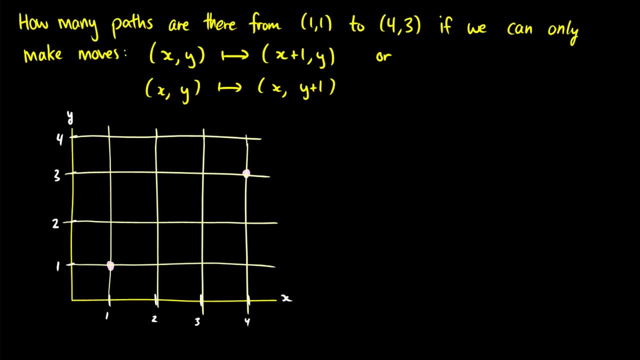 Now here's one more problem where we have permutations, but it's disguised as a graphical problem. So here's the question: How many paths are there from 1, 1 to 4,, 3, if we can only move right on a grid or up on a grid? 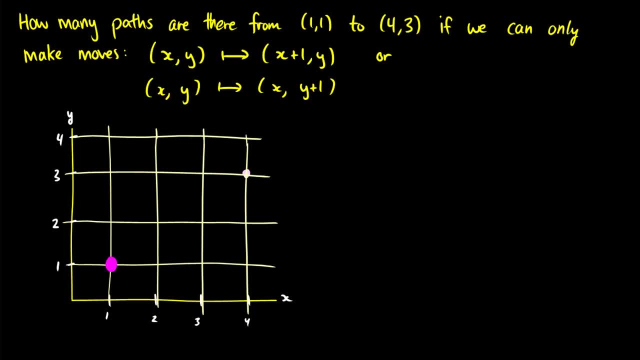 So here, visually, we're starting at the point 1, 1.. We want to end at the point 1, 1.. We want to end at the point 4, 3.. And we can either go up or we can go right. 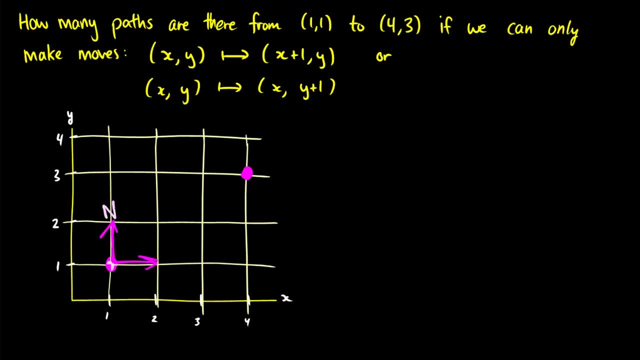 I'm going to give these specific labels. I'm going to say going up is called north and going right is called east. Okay, So what do we have to do to get from 1, 1 to 4, 3?? 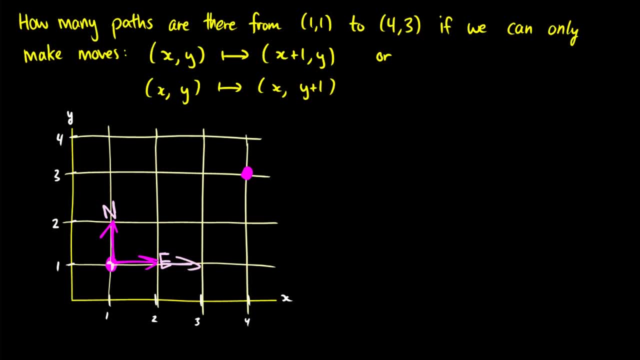 Well, we need to move right a total of three times. So we need to give ourselves three east movements. And we need to go up. We need to go up two times some time on our walk, So we need to give ourselves two north movements. 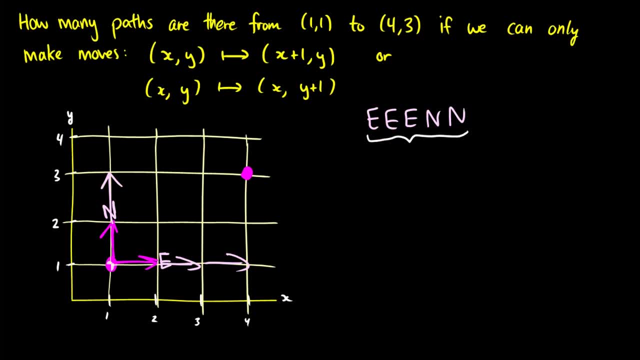 Okay. so, however, we can jumble these up. we can get a path from 1, 1 to 4,, 3.. And we can show this on the grid. So let's actually do this example. Let's get some random sequence like N, E, E, N, E. 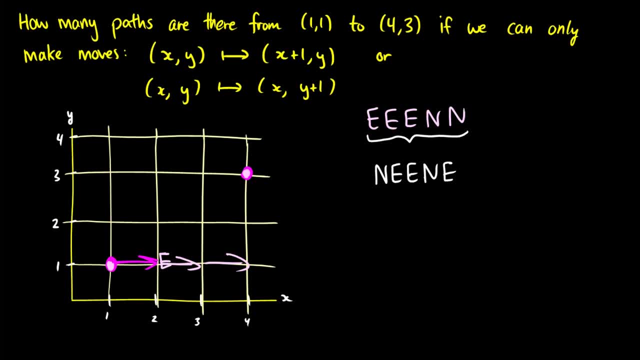 Okay, so we start at 1, 1.. So first we're going to go north, Now we're at 1, 2.. We're going to go right to 2, 2.. Right to 3, 2.. 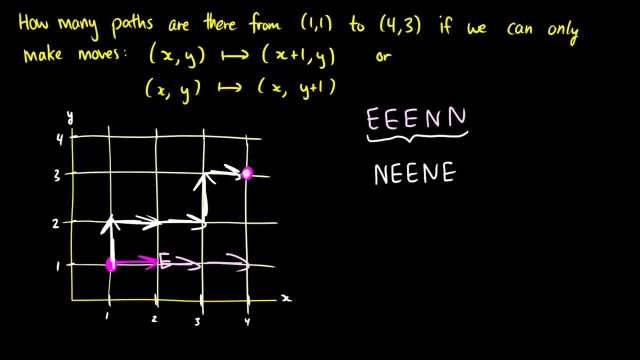 North to 3, 3.. And then east to 4, 3.. So that's one path. So really, this is just a word rearranging problem. There's five total letters, essentially Five total moves. Three of them are easts. 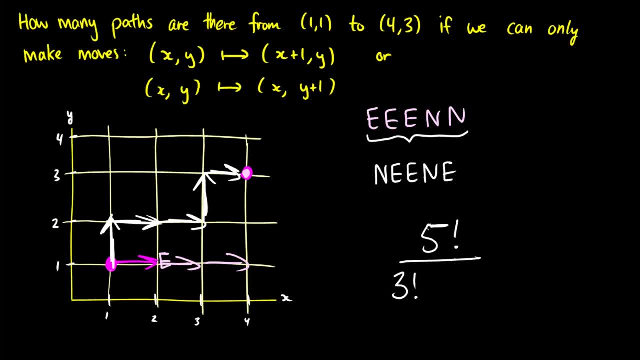 So we divide by 3- factorial, Two of those are norths. We divide by 2, factorial, And this is the number of ways in order to walk from 1, 1 to 4,, 3, if you only move right or only move up. 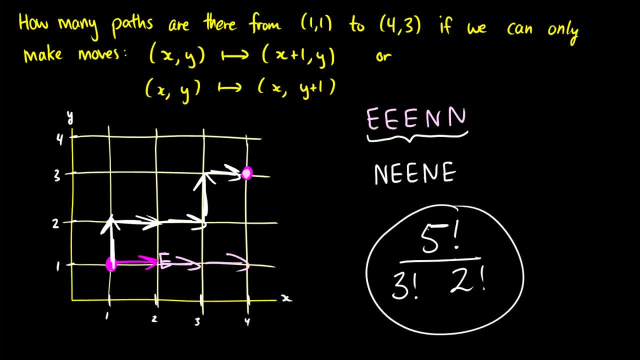 If you have any questions, please leave them in the comments below and I'll answer them the best that I can. 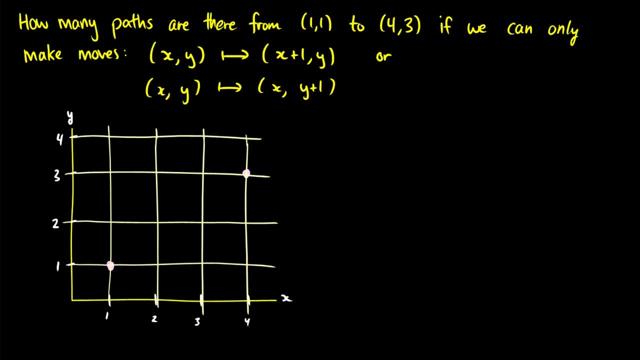 Here's one more problem where we have permutations, but it's disguised as a graphical problem. Here's the question: How many paths are there from one, one to four, three, if we can only move right on a grid or up on a grid? Here, visually, we're starting at the point one, one. 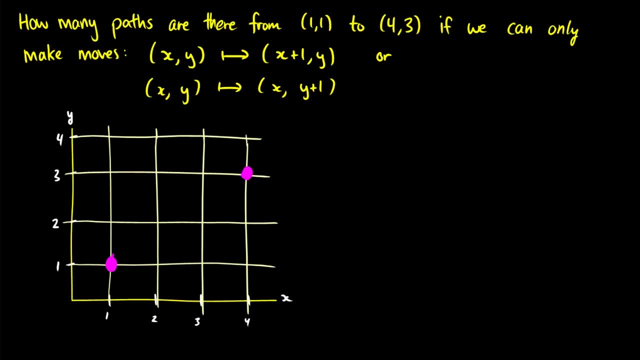 We want to end at the point one. one. We want to end at the point four. three, And we can either go up or we can go right. I'm going to give these specific labels. I'm going to say going up is called north and going right is called east. 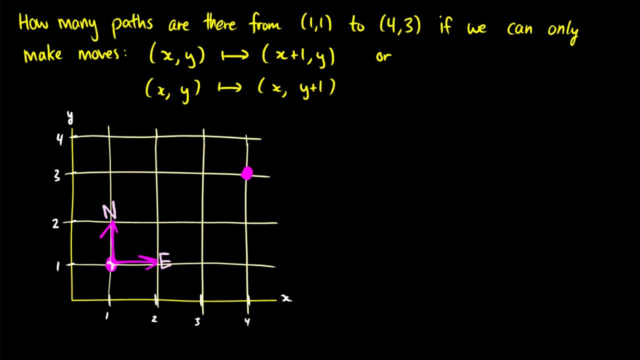 Okay. So what do we have to do to get from one one to four, three? Well, we need to move right a total of three times, So we need to give ourselves three east movements. Okay, We need to go up two times sometime on our walk, so we need to give ourselves two north. 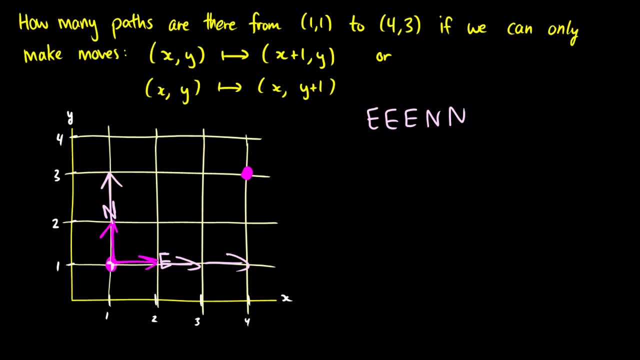 movements, Okay. So, however, we can jumble these up, we can get a path from one, one to four, three, and we can show this on the grid. So let's actually do this example. Let's get some random sequence like N, E, E, N, E. 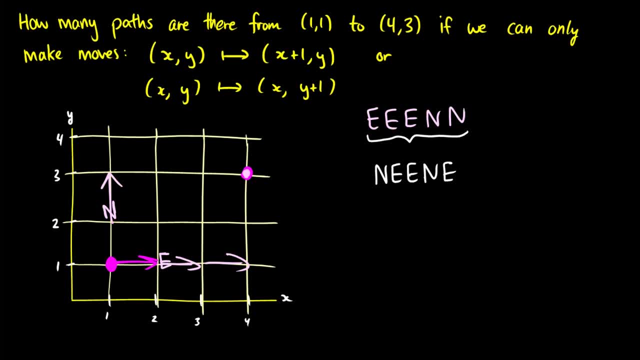 Okay, So we start at one one. So first we're going to go north. Now we're at one, two, We're going to go right to two, two, right to three, two, north to three, three, and then east to four, three. 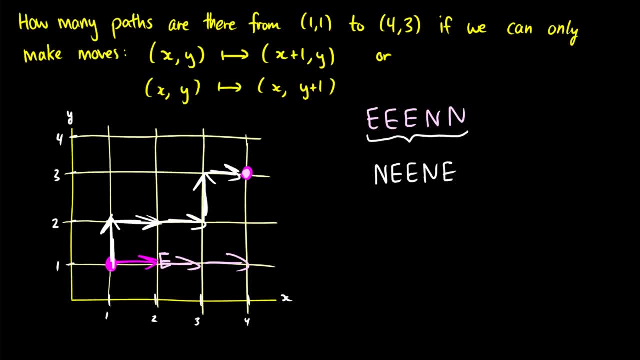 So that's one path. So really this is just a word rearranging problem. There's five total letters, essentially five total moves. three of them are east, So we divide by three factorial. Two of those are north, We divide by two factorial. 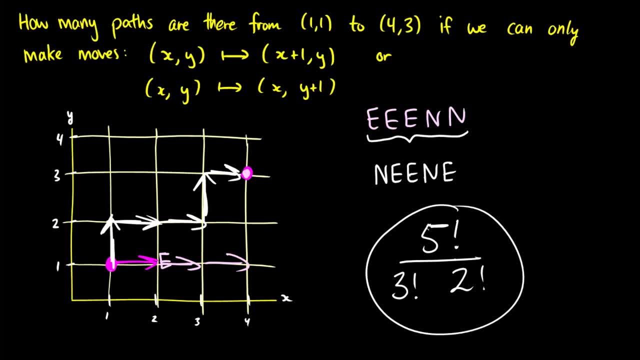 And this is the number of ways in order to walk from one one to four: three if you only move right or only move up. If you have any questions, please leave them in the comments below and I'll answer them the best that I can.